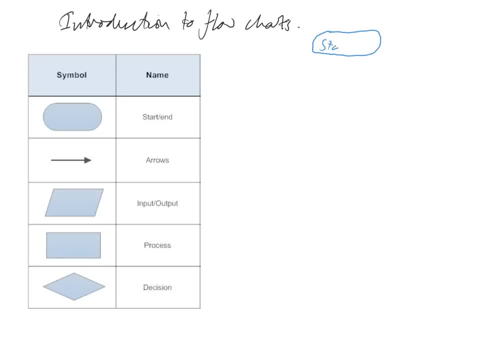 OK, this just signifies the start of our program. OK, we can then use an arrow Which shows Progress of the data through our flowchart. so I'll go there and the first thing we want to do is fill the kettle. now, filling the kettle is a process. OK, a process. 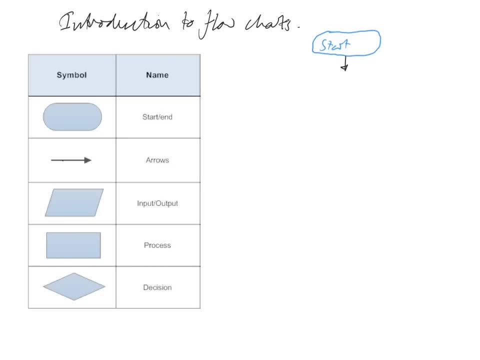 So it's a thing that happens in the program. OK, that's what a process is. So if I draw a rectangle, That's a really bad rectangle- And Fill Kettle do my best to squeeze my writing in here, and then we go down to the next part of the program. 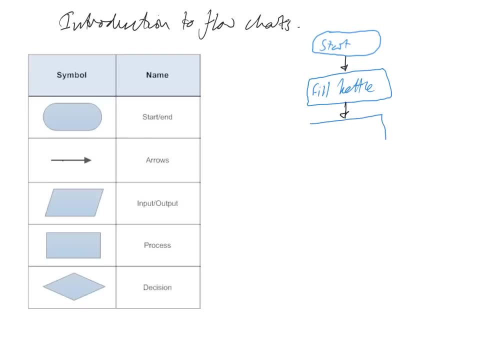 Which is another process. boil the water- OK, and then we go down to the next part of the program, Which is Get our cup and tea bag. Cup plus Tea bag- OK, and then we go to our next part of the process, which is a. 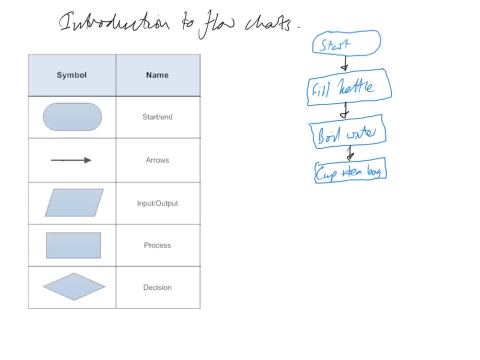 Boil the water, and what we can do for this is boil the water for two minutes, so we could make this a Decision box. OK, so boil water two minutes. okay, so, is the two minutes up? if it's not, we send our arrow back here. if it is, the two minutes is up, then we send our arrow onto the. 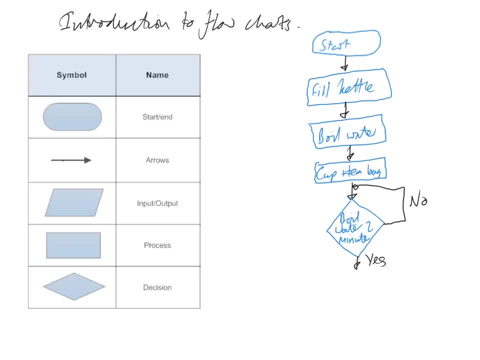 next process, which is take tea bag out. okay, out, there we go, and then add to milk. so again, this can be another decision. I'm not quite sure I'm going to squeeze this in. what I'll do, I think, is we'll just move on to the next.